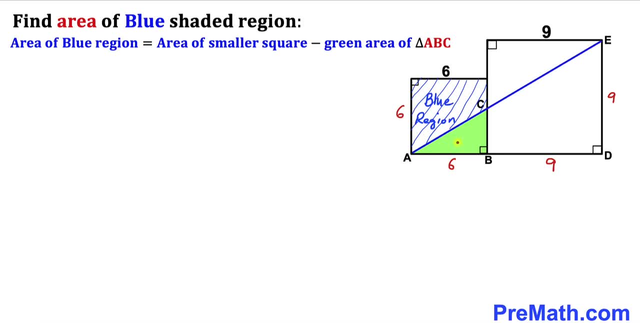 and calculate the area of this green triangle ABC. we know its base is six units. let me go ahead and call this height as X units. and now here's our next step. we can see that our this triangle ABC is similar to this bigger triangle Ad e, since this angle is 10. 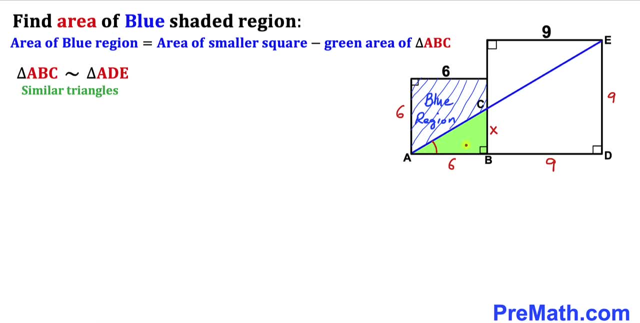 this angle is in common between both of them. these angles are 90 degrees each and these are their corresponding angles. so therefore we conclude that these two triangles are similar according to angle angle angle theorem. now we know that the side length of this smaller square is 6 units, so the length of this line, segment AD, is going. 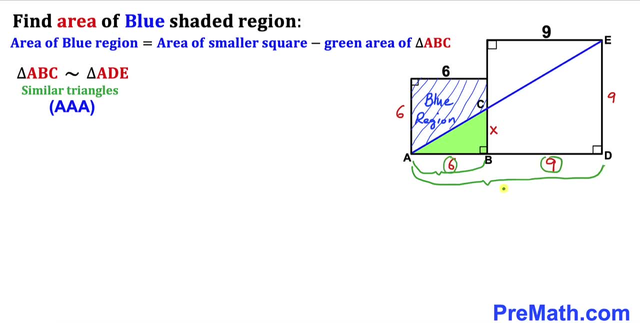 to be 6 plus 9 is going to make 15 units. so therefore we are going to have proportion. that means we are going to have a ratio of X divided by 6- let me go and write down X divided by 6: equal to this 9 divided by this big length: 15. let me go and write down 9 divided by 15. now let's go. 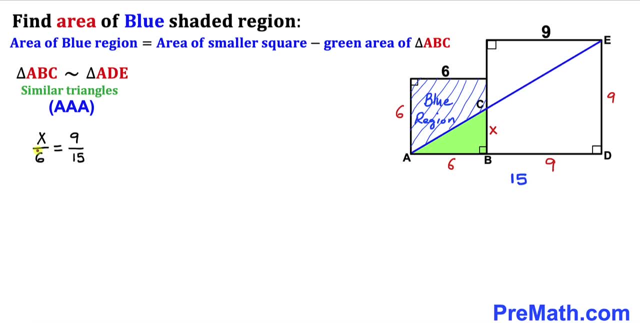 ahead and solve this equation for X. let me go ahead and remove this 6 from the denominator. by multiplying both sides by 6, we can see this 6 and 6 is gone. so therefore our X will be equal to 9 divided by this big length, 15. let me go ahead and write down 9 divided by 15. 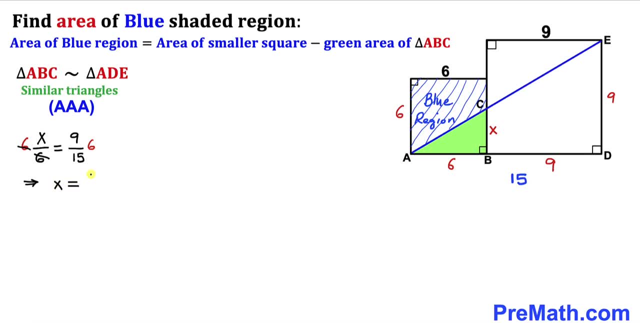 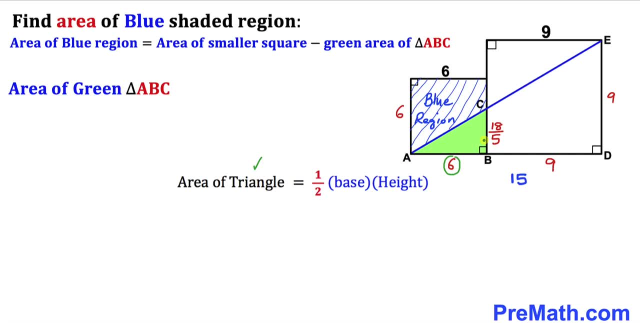 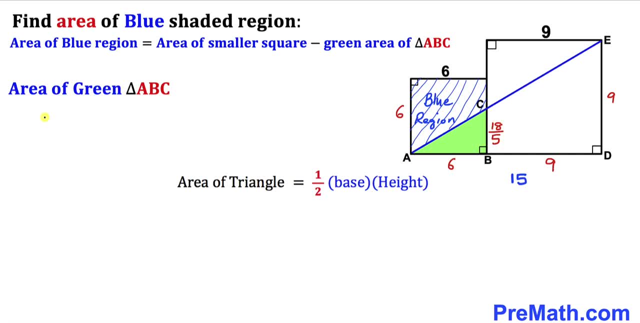 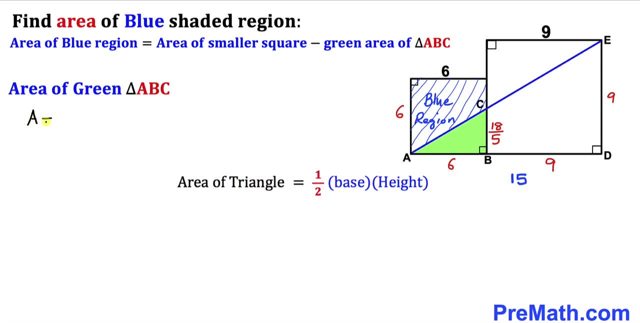 the area of a triangle formula area equals 5. and now let's recall the area of a triangle formula: area equals 5. and now let's recall the area of a triangle formula: area equals 5. and now let's recall green triangle: ABC turns out to be 54 divided by 5, or we can write this one: 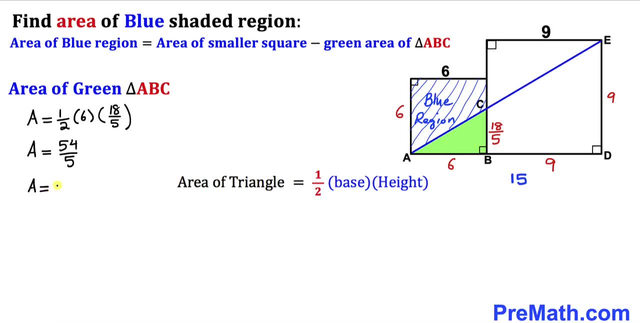 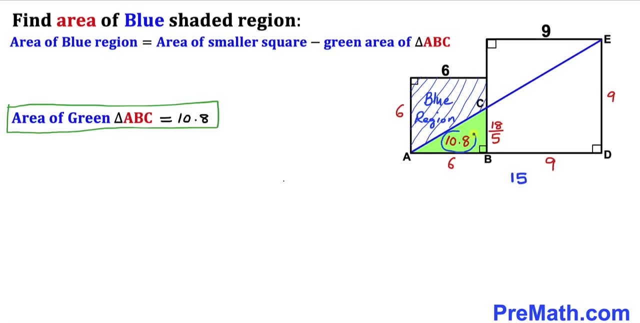 area equals to, in terms of decimal, 10.8. therefore, the area of this green triangle turns out to be 10.8 square units. now let's go ahead and calculate the area of this smaller square. now let's recall the area of a square formula: area equal to S- square, where S represents the side length of this. 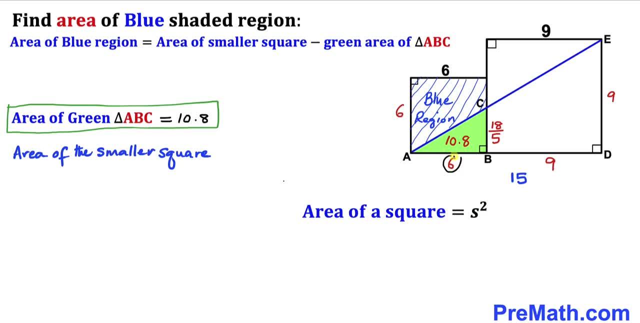 smaller square in our case is the side length is 6, so therefore the area of this smaller square is going to be 6 square. so that is going to give us 36 square units. and here's our final step. let's go ahead and fill in the blanks in. 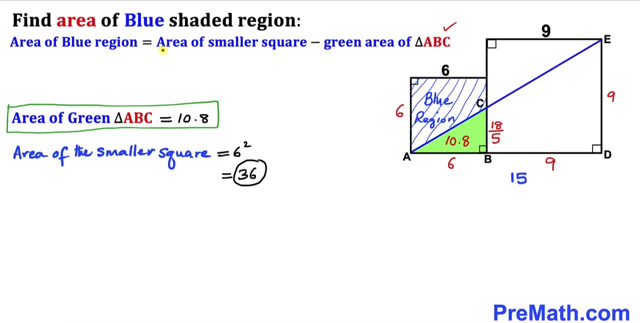 this equation, we know the area of this smaller square is 36 and the area of this green triangle is 10.8. so therefore, the area of this blue shaded region turns out to be 36 minus 10.8, and if we subtract this thing, that is going to give us 25.2 square. 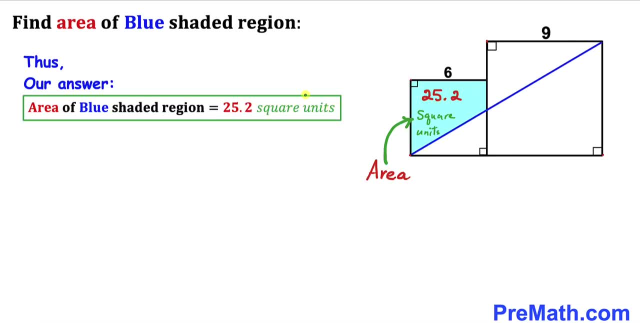 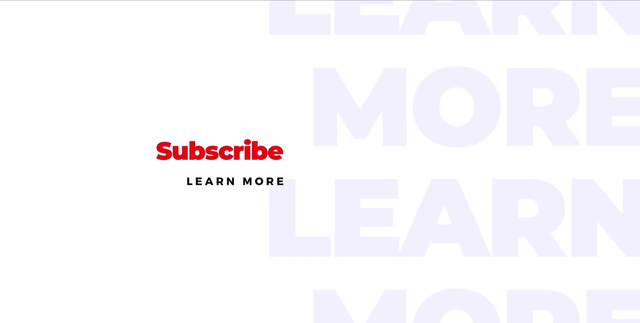 units. so thus the area of this blue shaded region turns out to be 25.2 square units. thanks for watching and please don't forget to subscribe to my channel for more exciting videos. bye.